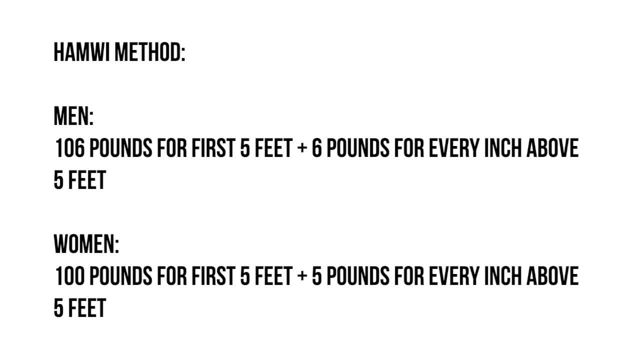 for males, it calculates the weight range by taking 106 pounds for the first five feet of their height and then adding an additional six pounds for every inch which is over five feet. For females, it calculates the target weight range by giving them 100 pounds for the first five feet. 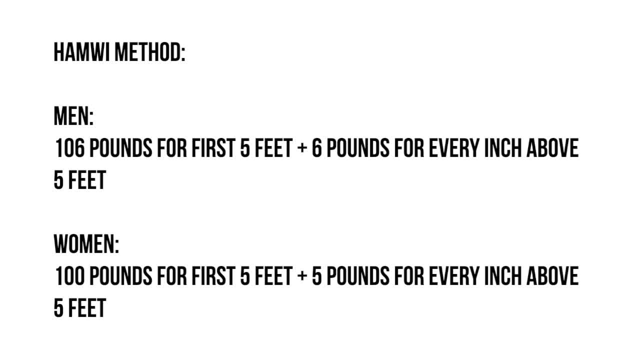 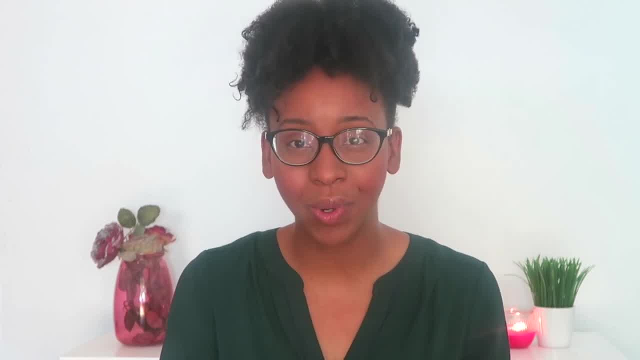 and then an additional five pounds for every inch above five feet. So it should be noted, according to the Academy of Nutrition and Dietetics Nutrition Care Manual, that the adjusted ideal body weight may overestimate or underestimate the resting metabolic weight. But for the purposes of the RD exam, this video and even your coursework I'm still going to show. 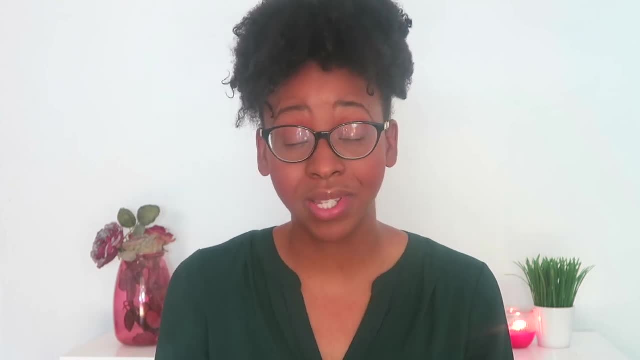 you guys how to calculate the adjusted body weight for individuals that do have amputations. So in my clinical practice the most frequent type of amputations I see are individuals that have an above the knee amputation as well as a below the knee amputation. So it should be noted. 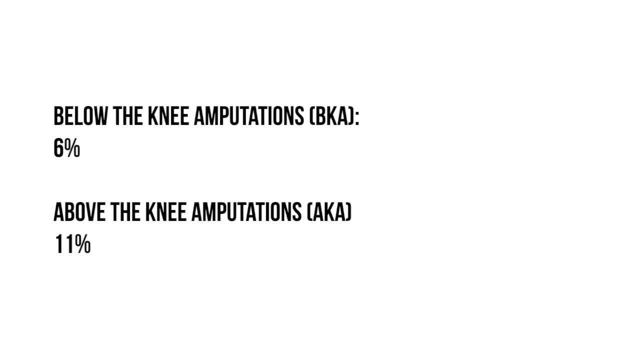 here and remember this because you're going to need this later on in the video. For below the knee amputation, that accounts for six percent of the body weight, and for above the knee amputations, it accounts for 11 percent of the body weight. So let's look at a quick scenario. You have a patient. 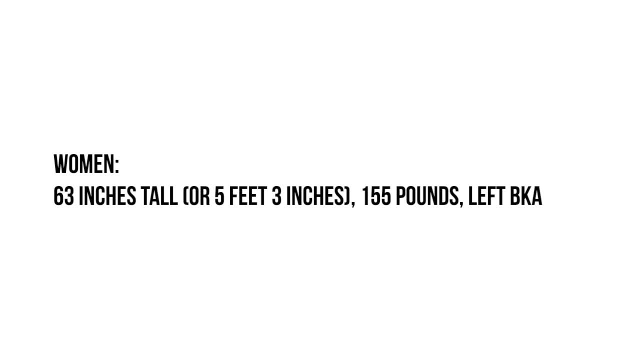 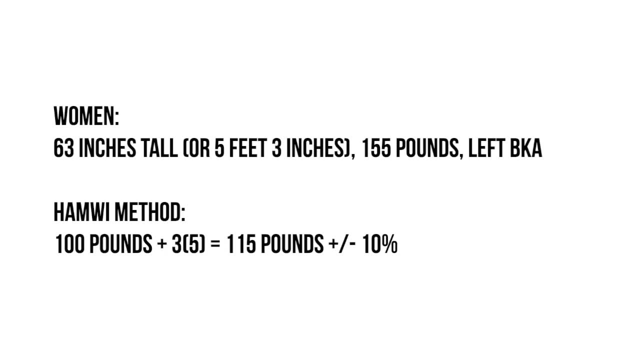 and she is female. We are told that she is 63 inches tall, weighs 155 pounds and has a left below the knee amputation. Using the Hamwe method, we are definitely going to give her 100 pounds because she is at least over five feet, and then for every inch below the knee amputation we are 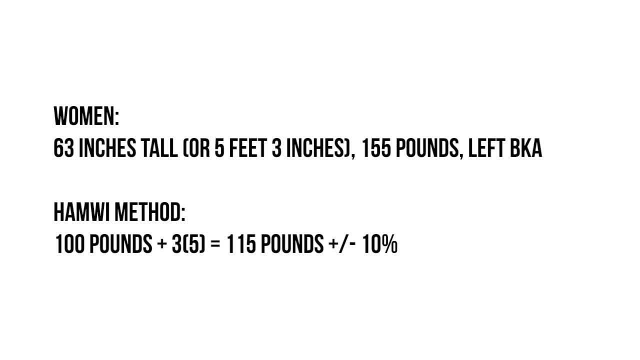 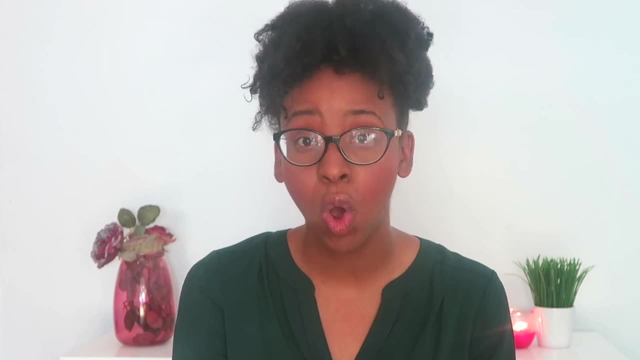 going to add an additional five pounds. So, using the Hamwe method, her target weight range is 115 pounds, plus or minus 10 percent, and the reason why there's that plus or minus 10 percent is because it takes into consideration if she has a large frame or a small frame. So then you want to use 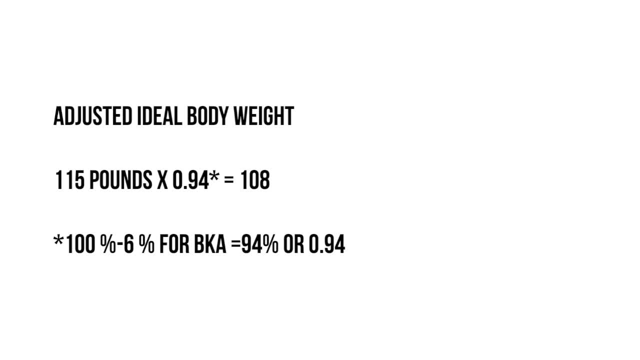 this 115 pounds to calculate her adjusted ideal body weight, based on the fact that she does have a below the knee amputation. So you want to take this 115 and you want to multiply it by 94.. The reason why you want to multiply it by 94 is because we were told that she has a left below.